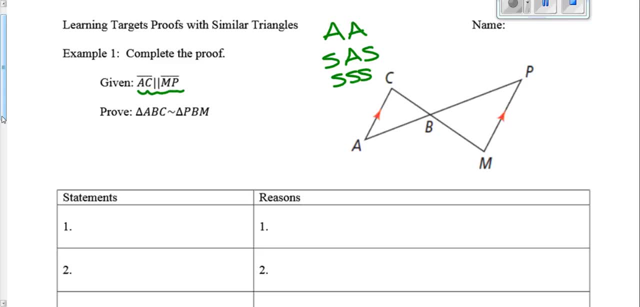 first. So the arrows proving parallel are already on our diagram. but what does it mean? What do parallel lines tell us? They give us congruent angles. Okay, so I'm going to go and mark some stuff. If these two lines are parallel, then I can. 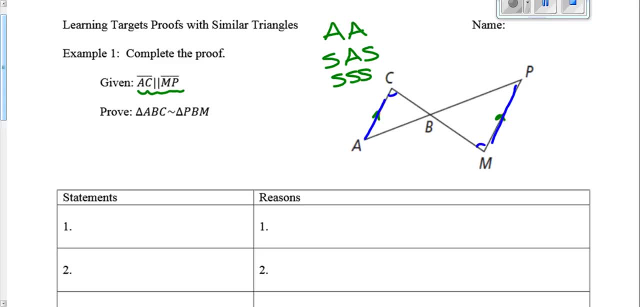 say that angle C is congruent to angle M, Why, They are alternate interior angles on opposite sides of this transversal down the middle. Okay, this guy right here. and they are on the inside of our parallel lines. I can also say that A is congruent to P. Okay, 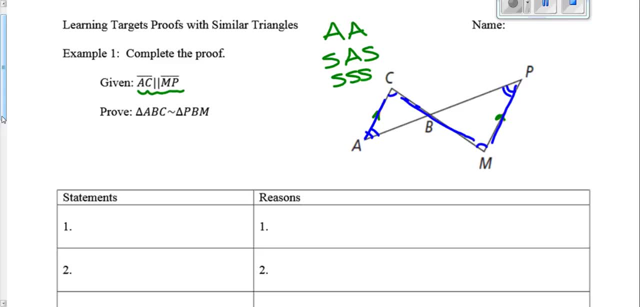 now, before we go on, what else can we conclude? I'm going to erase these lines right here. I know that, not only this right here, but I also know that these two are congruent right here because they are vertical angles. So always go to your diagram and see what information 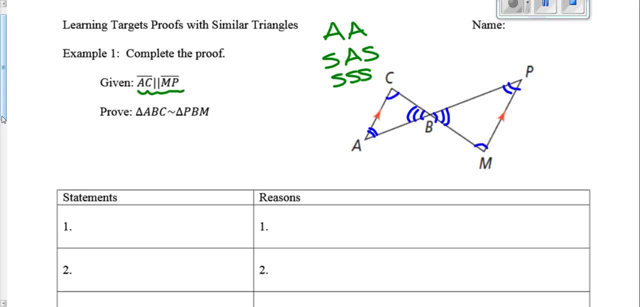 you can pull out first and use that to help you to prove similarity. Okay, now I only have three reasons to pull from: angle angle side, angle side and side side side. Well, look at it, All the information we're talking about is angles, so it makes sense that we 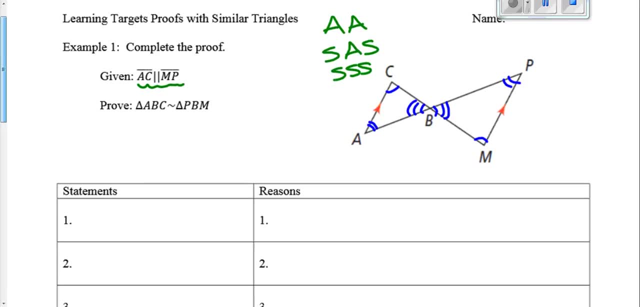 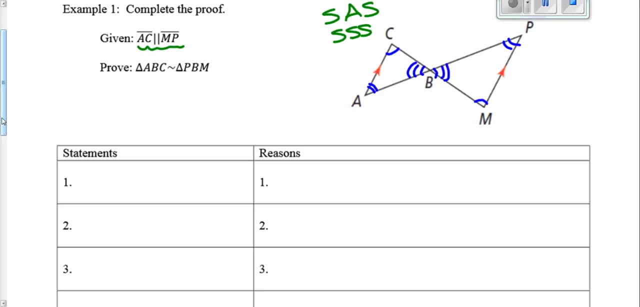 are going to use the angle angle postulate in this proof. Okay, let's start jotting stuff down. Also, it's important before you start to look at what triangles you're proving congruent. Here it's ABC and PBM. I'm going to outline them. 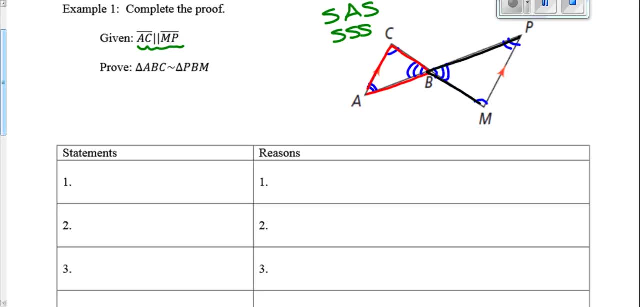 in different colors. Okay, because sometimes- you'll see in a further example- there's more than one or two triangles there, so you've got to make sure you know which one you're looking at. All right, so the first thing that we always write in is the given, So that 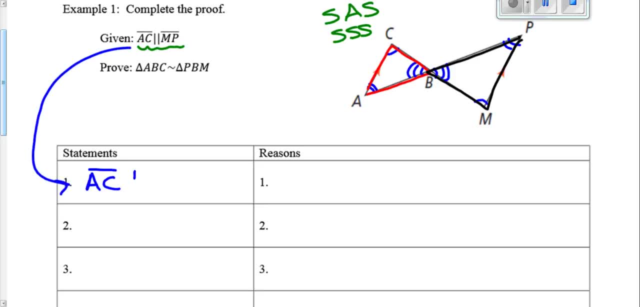 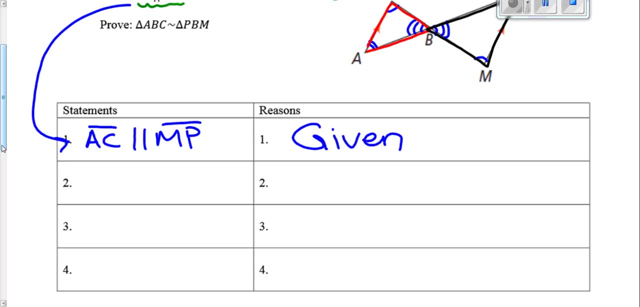 is going to go in step one. AC is parallel to MP Given. Well, we already talked about it and we know that we're trying to go with the angle angle postulate because we know nothing about side lengths. All right, so let's start out. 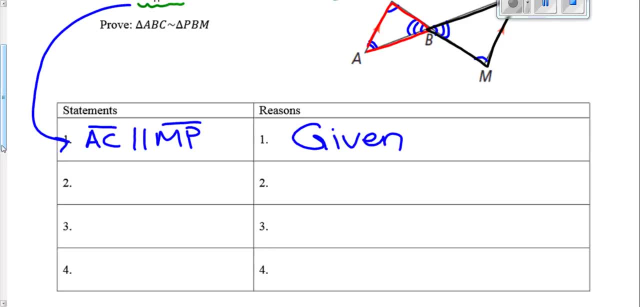 by now we have to make our statements. We need to prove at least two angles congruent, So let's start with the vertical angles. Okay, so I have angle ABC and that is going to be congruent to angle PBM. 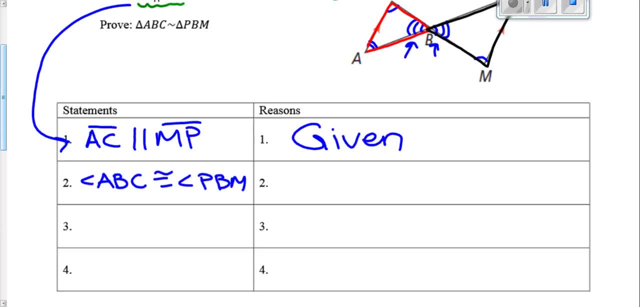 Okay, so these right here, and the reason for that is vertical angles. So what we again are doing in the statement column is listing the congruence or the proportional side lengths, if that was happening in this picture. this not Okay, so we need to write. 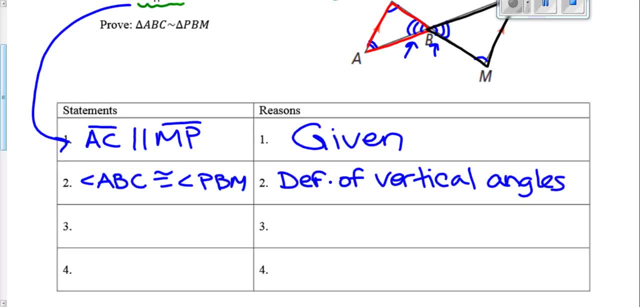 down all this information, All right. and then I can also say that angle C is congruent to angle M. I also can say: angle A is congruent to angle P. Now, I do not need all three angles, okay, I do not need to prove all three, I only need two. But I know that both of these work because 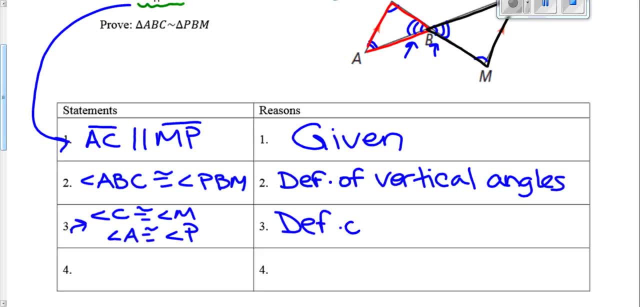 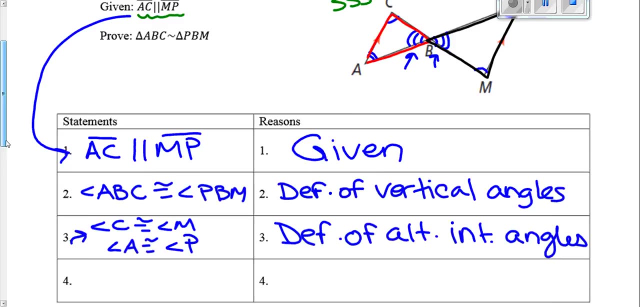 we're also at interior, So let's come back to that thought in a second. really, I can do a vertical angle and then one of the alternate interior angles, because I don't need to list all three, or we could have cut this proof down by one step and we could have cut out line. 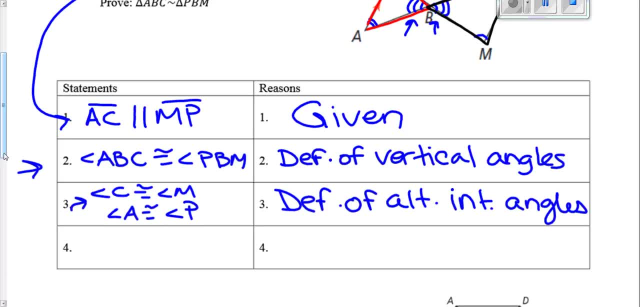 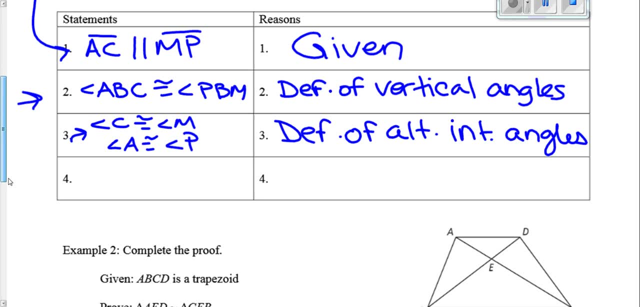 two, we don't need the vertical angles because we only need two angles, and when I have parallel lines cut by transversal, I get two sets of alternate interiors. so just something to think about. all right, my last step: I have my angles in there, so make sure that you have enough information. 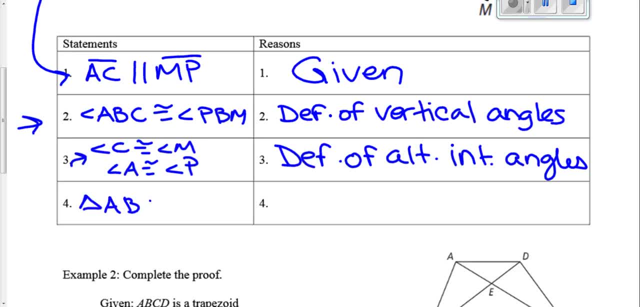 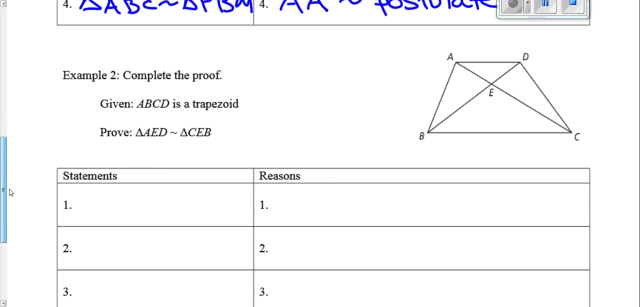 and I can say that triangle ABC is similar to triangle PBM. why our angle? angle similarity postulate: all right. so angle angle: if you need to pause the video, rewind and go back and watch that proof again, all right. number two: given ABCD is a trapezoid, we are proving AED is 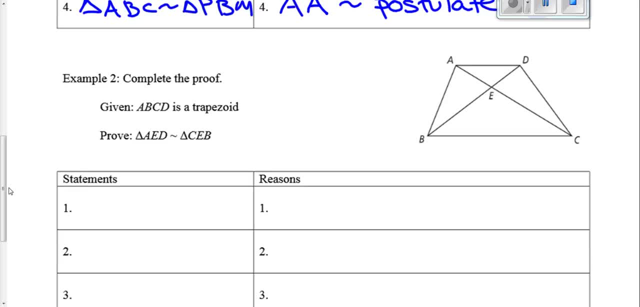 um, similar to CEB. all right, here's an example where you have quite a few triangles, so I'm going to highlight AED. it's off a little, but you get the idea. and then this one down here, so we know which two we're looking at. okay, now, before we get started with the given, what do? 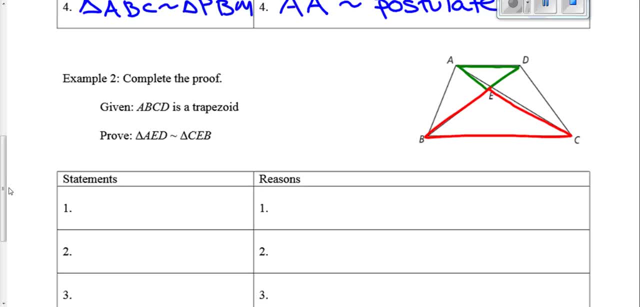 we already notice. if you said vertical angles, you are correct. if you notice that my lines are off, that's not helpful information. all right, so I vertical angles. okay now, ABCD is a trapezoid. remember, if you're given something, it's for a reason you. 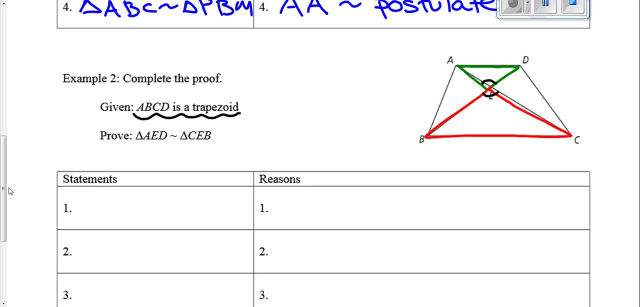 learned about trapezoids way back in the day in middle school. you may or may not remember, but in a trapezoid line A, D are two bases, so AD and BC are parallel. okay, I'm just going to jot down that down right here. AD is parallel to BC. we'll talk about that in a minute and how. 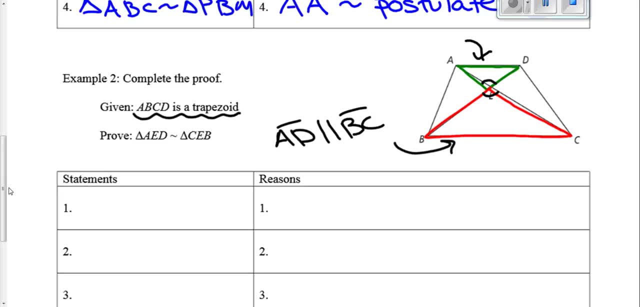 to put that in our proof. but will you parallel lines apply alternatives? what I have here is alumni alternate interior angles, so once again I can say D and B and then this one with this one okay. so once again I'm looking at angles, not sides. so this will be an 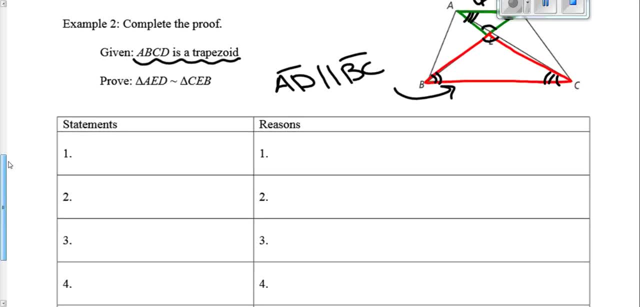 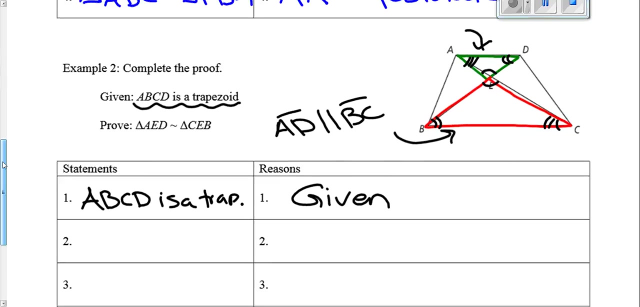 angle, angle postulate: okay. so let's talk about our reasons in our statements. first of all, given always trap. okay, now we can just go ahead and state our vertical angles, because that's something that we don't need a given for its truth anytime things cross each other. so, looking at our diagram, we have angle a. 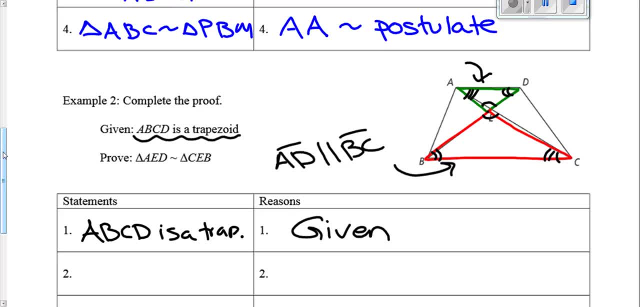 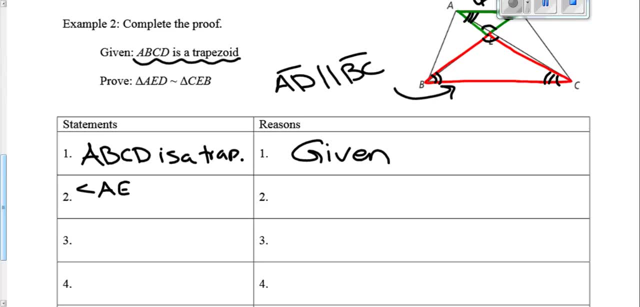 ed is congruent to C, e, B. why definition of verticals? all right, now we're going to go back and we're going to pull up the other angles, but we need to state this statement right here. okay, we're given that it's a trapezoid, but what is a trapezoid imply? it implies 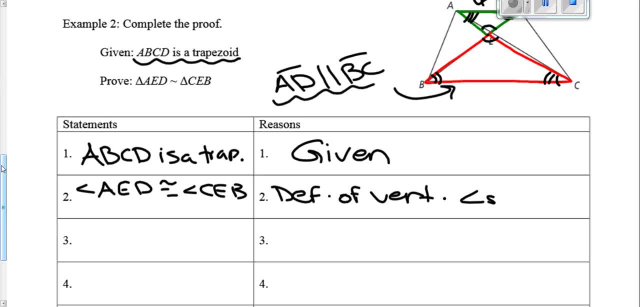 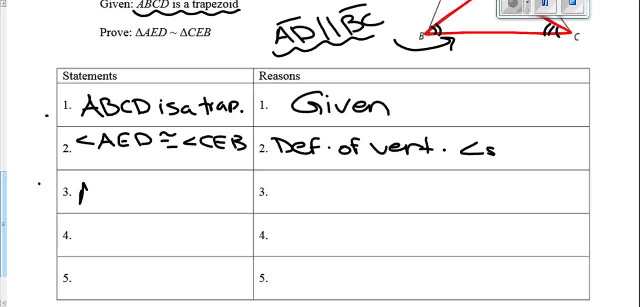 parallel lines, which thus then implies angles. so we have to provide every step. so here we're told it's a trapezoid. so down here we're going to write that parallel statement. ad is parallel to BC. why? all right, we can say definition of a trapezoid. we can say on basis of a trapezoid or parallel. 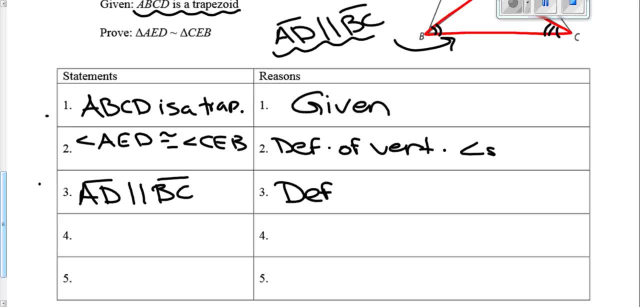 however you want to word it, but knowing that trapezoid implies that okay. so if you write something in your proof once again, it is for a reason. why did we write that? we wrote that so that we could say that our trapezoid is a trapezoid. so we can say that our trapezoid is a trapezoid. so we wrote that so that we could say that our 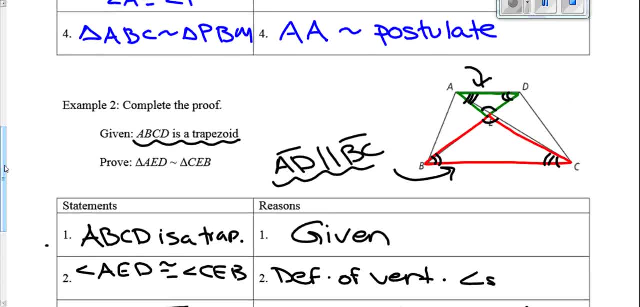 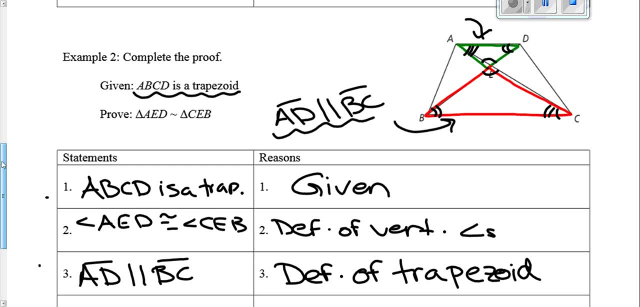 angles were congruent. okay, once again, I don't need both of the angles, both of my alternate interiors in this case. I'm just gonna write them both so we can see it. but keep in mind, we only need two sets of angles, so we could have really. 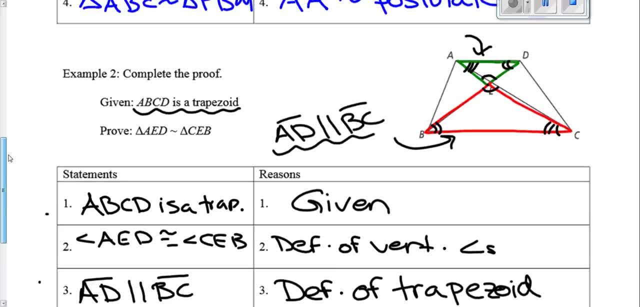 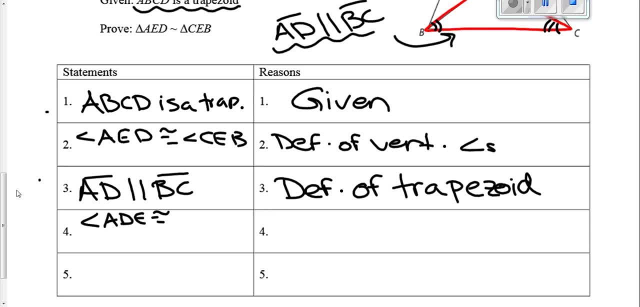 taken out. step two, if we wanted to, all right. so here we go. we're gonna write our angles in. angle ade is congruent to angle CBE, all right. and then angle dae is congruent to angle bce. why alternate interior angles? all right, we. 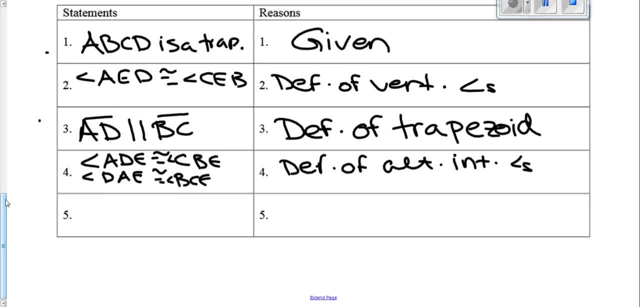 have enough information to now conclude. the triangles are similar, so triangle a e D similar to triangle ceb. angle-angle postulate. Notice we're saying similar here because it's not congruent, so you need to state it's an angle-angle, similar postulate. Alright, first step should always: 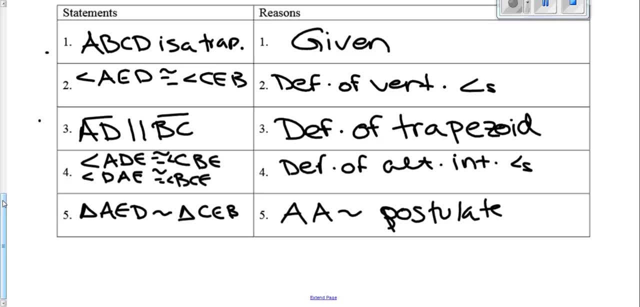 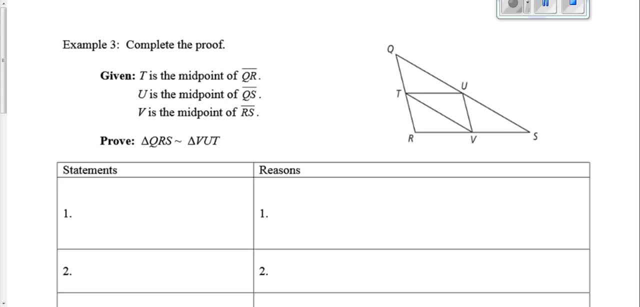 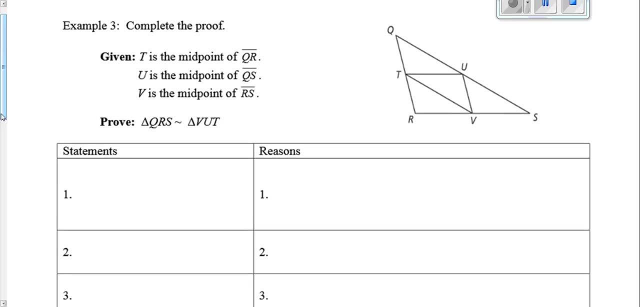 match your givens. Last step: what you're proving Once again, pause the video, go back if you need to see this proof again. Alright, now this next proof. we are going to be learning a new concept in here, so make sure that you are really paying attention. So we're given. 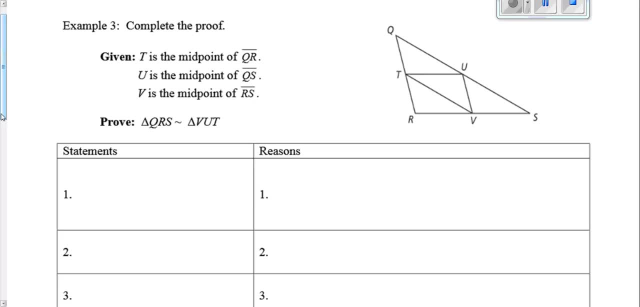 that T is a midpoint of QR, U is a midpoint of QS and V is a midpoint of RS. Alright, what does midpoint imply? It implies that it's cutting a diagram in or, I'm sorry, a line in half. So if T is a midpoint of QR, that tells me that these two little line segments 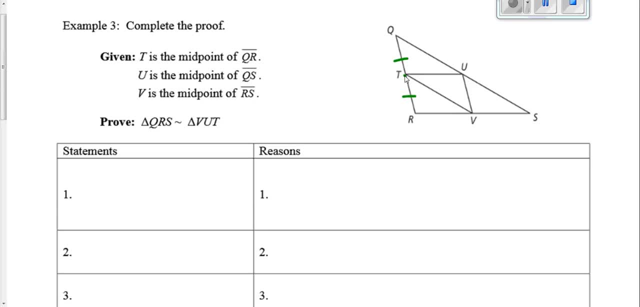 are the same length. Alright. then it tells me that U is a midpoint of QS, So these two are the same, And, last but not least, V is a midpoint of RS, so these two are the same. Okay, now let's take a look at what we are going to prove. Alright, I don't have any angles. I. 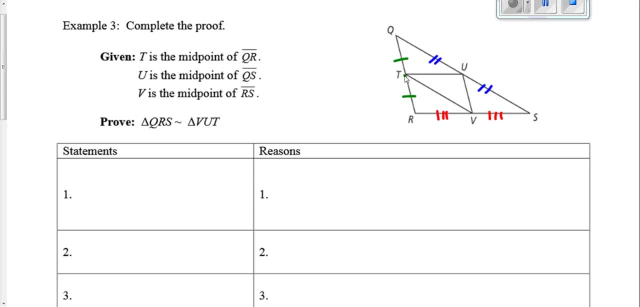 can do here. There's no verticals, there's no shared angles. Okay, so we're proving that QRS is similar to VUT. so let me draw that QRS is the big guy and UVT is this little guy. I'm going to make him in a wavy line. 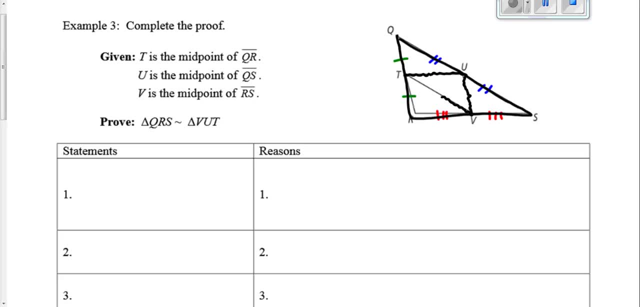 So you're going to see the difference between the two. Okay, So, once again, no shared angles. So clearly, the only thing we're looking at is sides. Okay, I don't have any vertical angles. like I said, I don't know any parallel lines, so I'm not going to grab any alternate. 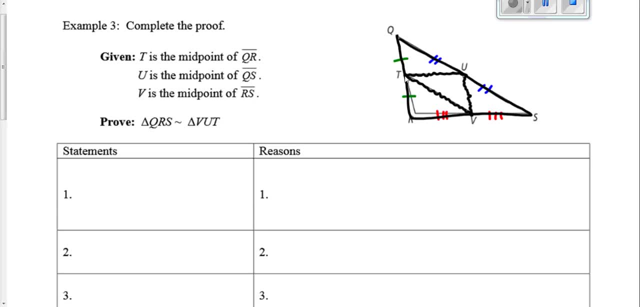 interiors. Okay, no corresponding. So therefore, it's probably going to be a side-side-side postulate. So let's look at it. Given the information we have and the markings that I made, how is that going to help us say that QRS is similar to VUT? 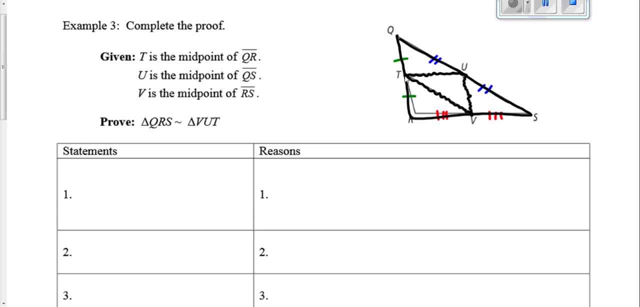 based off of that, it's not going to. okay, I can't conclude anything based off my markings. okay doesn't meaning it doesn't matter to me that those two are equal, because that's not both. these little halves are not part of the little triangle in the middle. all right, there are true. 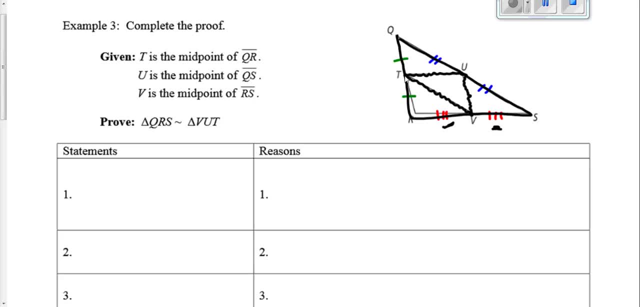 facts, but they're not going to help me. so here's what's going to be new. so let's go ahead and, everyone, let's write the givens in. so fill in all this information, please. while I write it, too, you do as well. how's everyone's night going, having fun doing math? 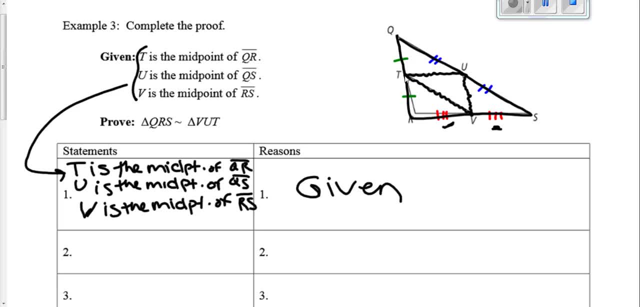 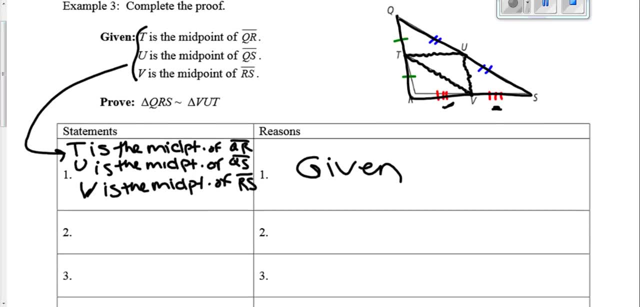 okay, so if you need more time, pause it so you can write it and then move on. all right, my givens are given to me now. here is what happens, and this is a new fact, so you probably don't know this, and that's okay. take a look at line ut, or to you. this line right here is one half the distance of rs. 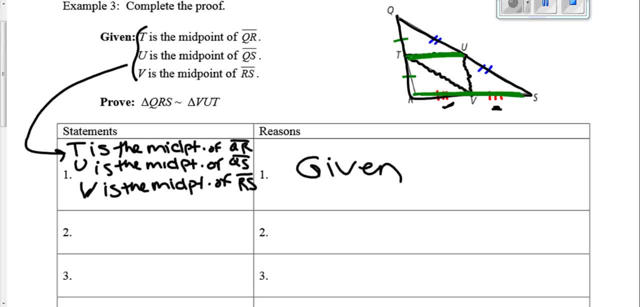 okay, why? because of this? because the fact that t is a midpoint of a line and the fact that u is the midpoint of another line, that means that the line that those two midpoints form is one half of the third side of the triangle. likewise, uv is formed by the midpoint u. 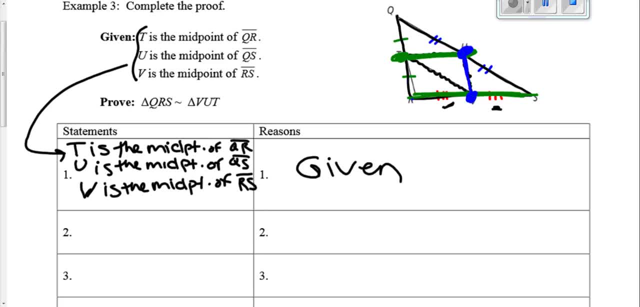 and the midpoint, v. so therefore uv is one half the distance of this guy. and, last but not least, t v, which you probably all rather be watching right now. t and v are midpoints of two lines of the side and the side or the line that they 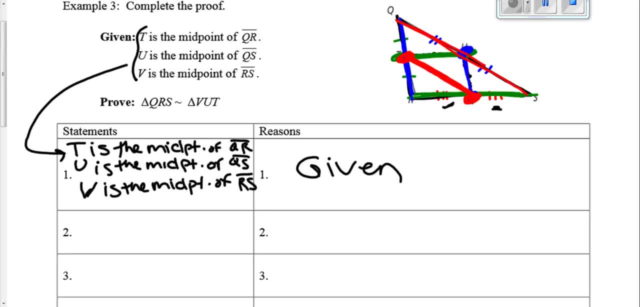 create is half the distance of this line right here, the other side of the triangle. it doesn't have a midpoint on it. so, that being said, my little circle in the middle, the red, green and blue one, this little guy right in here, all the sides are one half the distance of the outer. 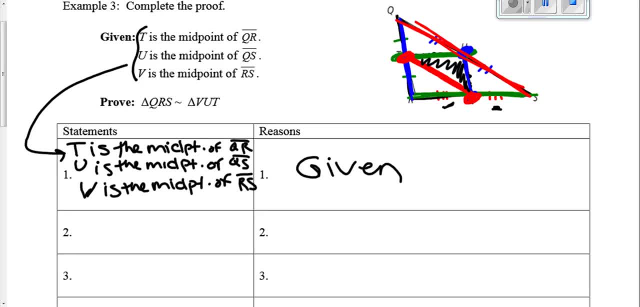 sides of the big triangle. so that means if they're all one half of the distance. if i were to tell you that this guy was ten, the other green one would have to be half that five. right, and i'm just making up numbers so you can see it. if i tell you that the blue 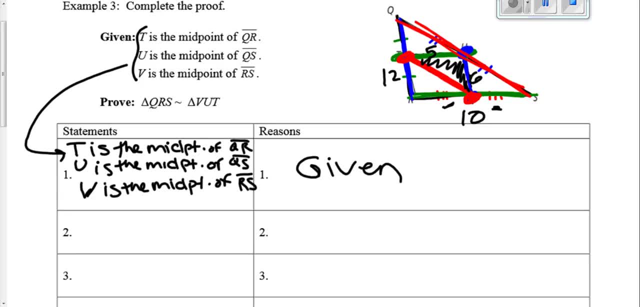 one is twelve, the other blue one, has to be six, one half the distance. if i tell you this one is twenty, this one is ten. so that means that the sides are truly proportional, so we can conclude a side side side here. that is the new fact that we are working with okay. 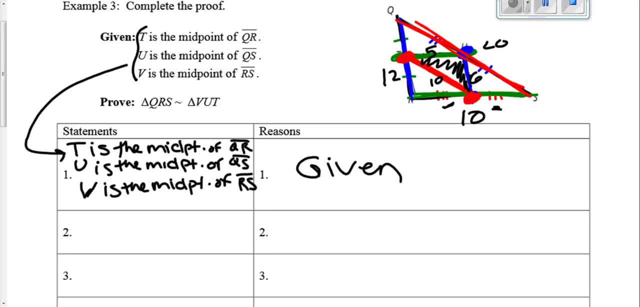 all of the sides of the little guy are one half the distance of the corresponding um. yeah, the corresponding sides of the bigger triangle. okay, and that is because they were all formed by midpoints, not just doesn't happen in any triangle, because this red line right here was. 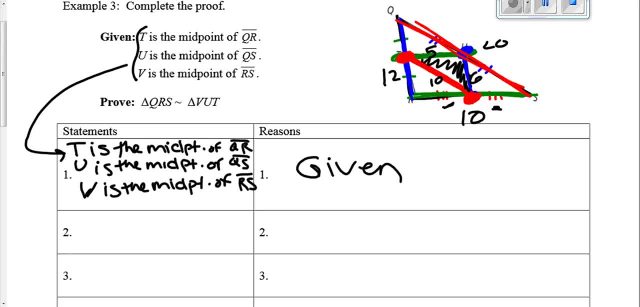 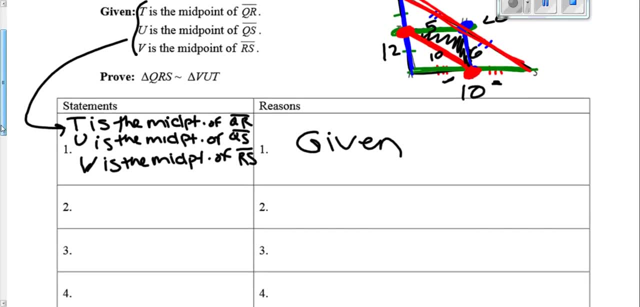 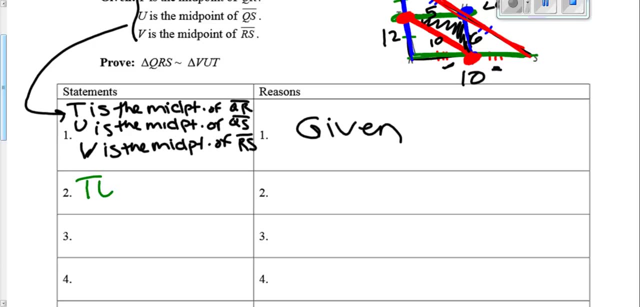 formed by two points that are midpoints of the other two sides of the triangle, so let's figure out how to write this in. ok, let's start with the green line, T? U. all right, so T? U, and I'm not putting a bar because we're talking length now is: 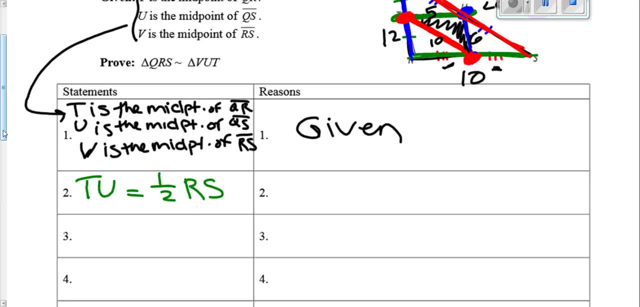 one half the length of RS. and remember we learned in unit one, we say length without putting the bar. that means length. ok, here is why the segments. so this is how we're going to word it: the segments connecting the midpoints of two sides of a triangle. 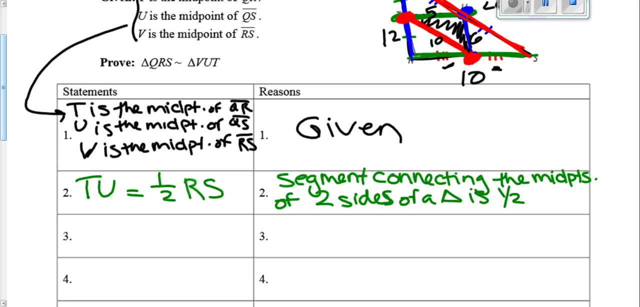 is one-half the base. alright, the segment that's connecting the two midpoints, the screen when I here it's connecting these two midpoints is one-half the distance of the base, meaning the other side of the triangle that doesn't have the two midpoints on. 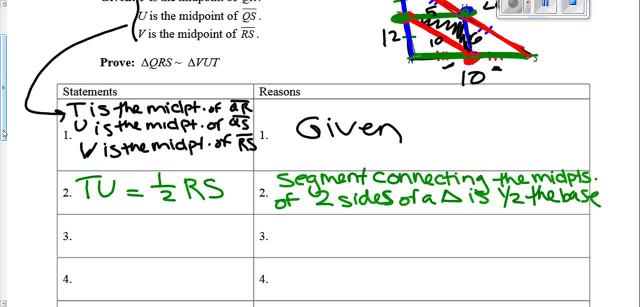 it. ok, now i'm going to write the same reason for the next two. so if you want to pause the video, I'm going to put a to go ahead and pause it and write it in, just to save a little bit of time. So you can pause. 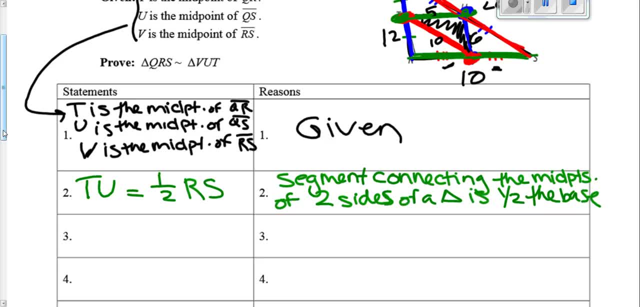 it too and write them in on your own. So the reason it's going to be the same for 3 and 4, I'm just going to have to use different lettering. So try to come up with these on your own- the sides that we're talking about. Okay, so I just paused it to fill in that. 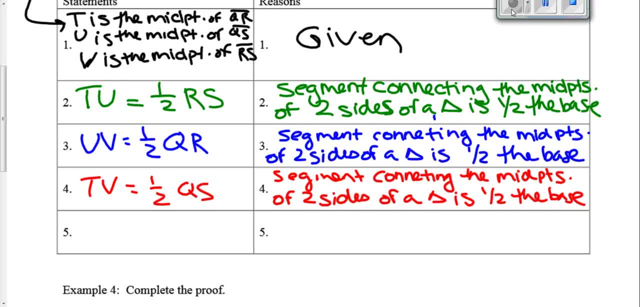 information. So UV is 1 half QR, the distance, and TV is 1 half QS. Okay, so, with that being said, I can now conclude that the two triangles are similar because of the side side side postulate, because all the sides are proportional lengths. We don't know what they actually. 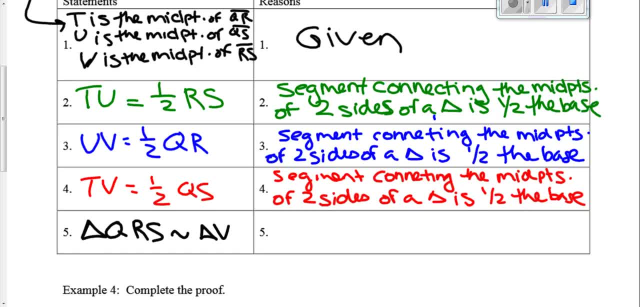 are. The numbers I put in were just to help you visualize it. but we don't really care, We just know that it's true. So, side side side similarity postulate: Okay, pause the video, go back, rewind if you need to. You're going to move on to the last example, So the 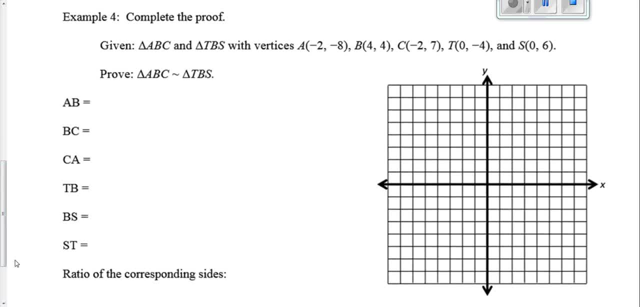 last example is doing a proof on a coordinate plane. So we're given triangle, ABC and TBS with a given vertices and we have to prove the ABC and TBS are similar in similar. So, guys, if it's on a coordinate plane, think for a second. what postulate do you think? 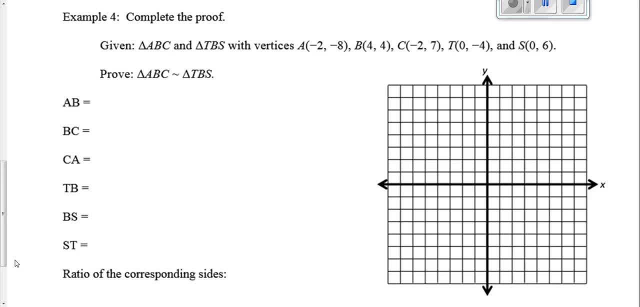 we're probably going to use. If you thought to yourself, it's side, side, side, you are correct. All right, because we're not really talking angles here. We know on a coordinate plane how to find the length. Okay, so we're going to use that side, side, side length. 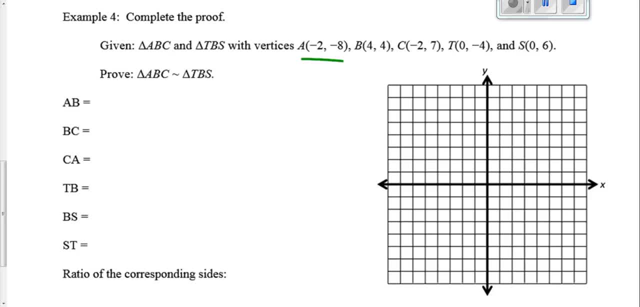 Okay, so let's go ahead and plot our points. A is at negative, 2, negative 8.. Negative 2, negative, 7.. 1,, 2,, 3,, 4,, 5,, 6, 7, 8.. Wait a minute, All right. B is at 4, 4.. 1,, 2, 3,. 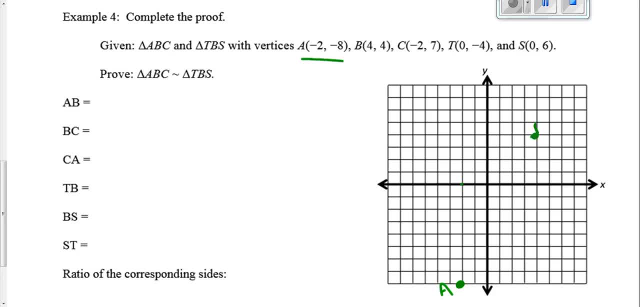 4, 1,, 2,, 3,, 4.. So you can be doing this with me, You don't need to just be watching. Negative 2, 7 is here, All right now. my other triangle I'm going to do in a different color, T is. 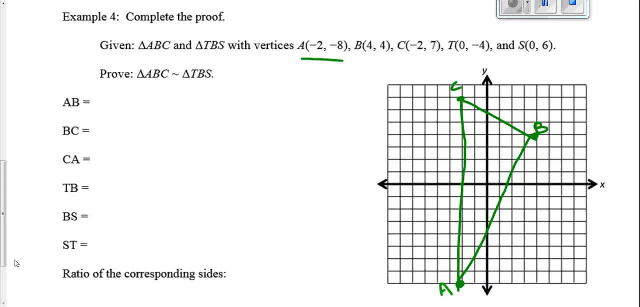 0, negative 4, it has the same point B, okay, because I'm doing TBS, so TB, and then S is at 0, 6, which is right here, right: 1, 2, 3,, 4, 5, just kidding, right here, okay, so. 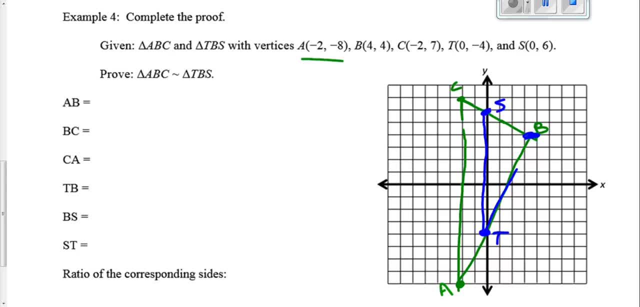 here's my smaller triangle, so we want to prove that these two are similar. okay, ABC and TBS. now just find the lengths of the sides, let's see if they're proportional. okay, so pause the video on your own, find the length of those sides, you guys should. 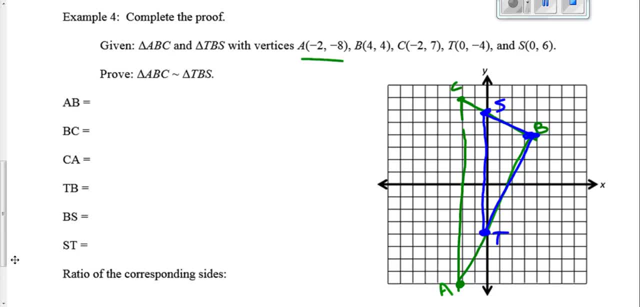 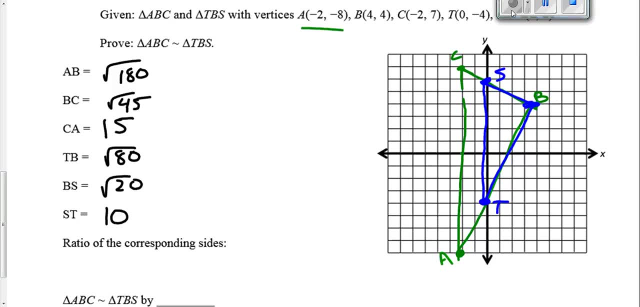 be pros at length by now. if you're not, you need to be coming in for practice, because at this point we expect you to be able to do it on your own. so pause the video. all right, match up your lengths with mine. if you got something wrong, try to find your. 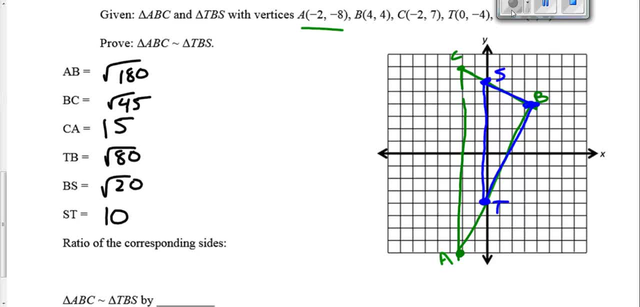 mistake. if you're not sure, once again, you need to be coming in for help. All right, so if I'm going to be proving that these two are similar by side side side, I need to find the ratio of the corresponding sides. so I know that AB and TB correspond.